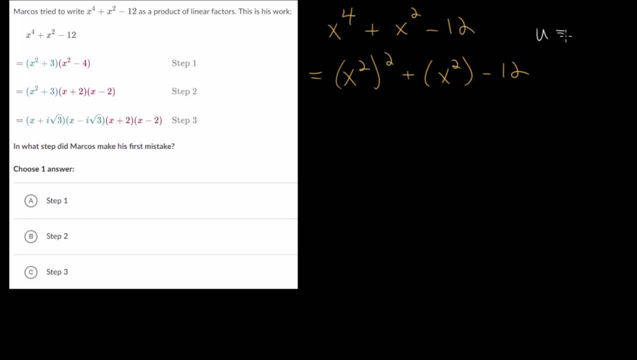 make a substitution. We can say that u is equal to x squared, so that we get u squared. Let me actually remove that parentheses. We have u squared plus u minus 12. And by transforming this using this substitution, u is equal to x squared. 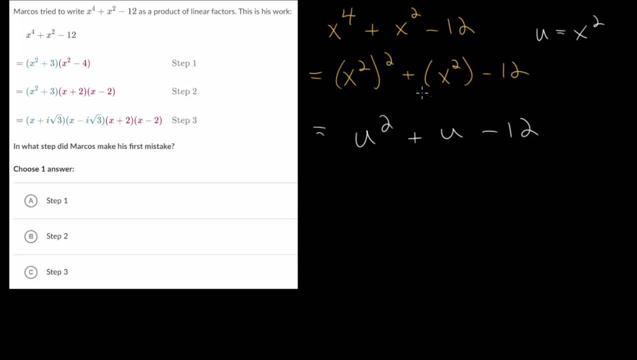 this now becomes a quadratic equation, And we can factor this using the techniques that we've learned for factoring quadratics. So let's start by writing this as a product of two binomials, And if this didn't work, then we can factor this using the quadratic formula. But let's see if this 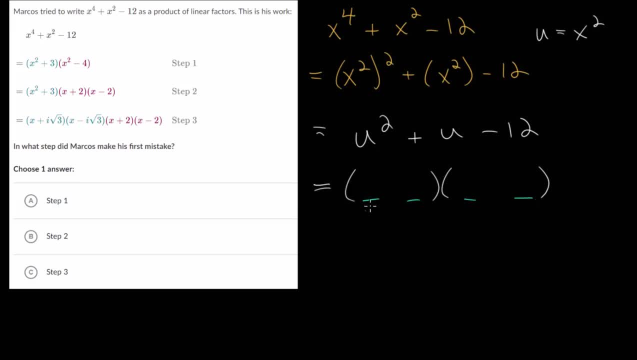 does work, Since we know each of these will have two terms. the first term in each would have to be u, Since if we rewrote this, we have u squared plus u squared, And if we rewrote this, we have u squared. 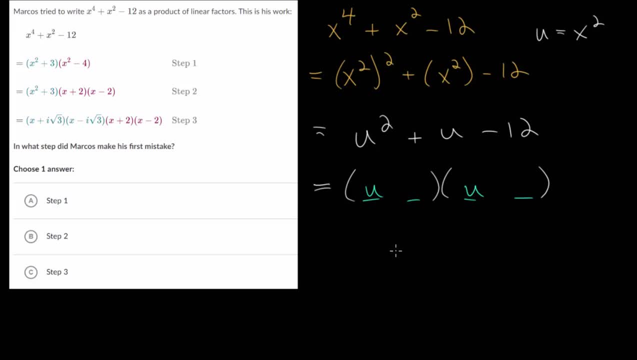 plus u squared, And if we remultiply it out, at the end u times u gives us u squared, And this term and this term here have to multiply to negative 12, but add to the coefficient on u, which in this case is positive 1.. So let's think about which numbers multiply to negative 12 and also add to. 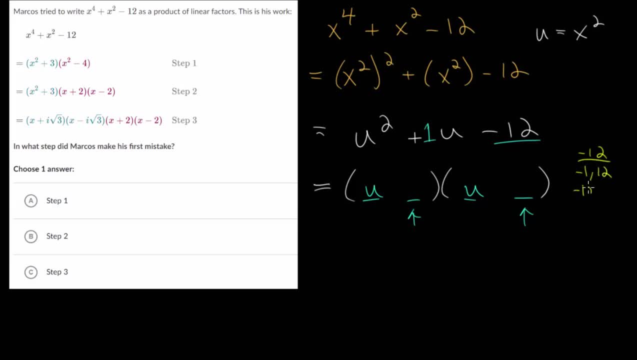 positive 1. We could have minus 1 and 12, minus 12 and 1. We could have minus 3 and 4, or minus 4 and 3.. And we can stop there, since we noticed that minus 3 and 4, if you add those together. 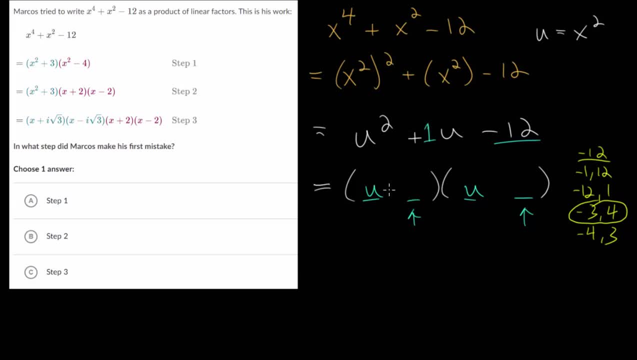 you do get positive 1.. So we can factor this as u minus 3 multiplied by u plus 4.. But we originally started with the variable x, so let's plug x squared back in for u, And by doing that we would end up with x squared minus 3 multiplied by x squared plus 4.. And at this point, if we go, 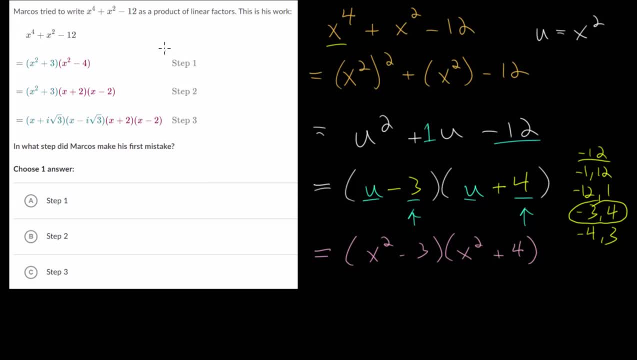 back and compare our work to his work, we can see that through step 1, we ended up with different solutions, So there's already a mistake here. In fact, notice that, compared to our work, the signs are switched. here We had x squared minus 3 and x squared plus. 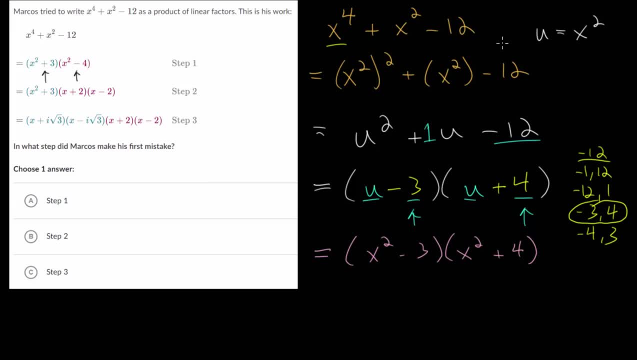 4.. And an alternate strategy, rather than working it out yourself, is that at each stage you can just re-multiply this back out and make sure that you get back the original expression, Since if we carried out distribution here, notice that x squared times x squared, that is x to the fourth. 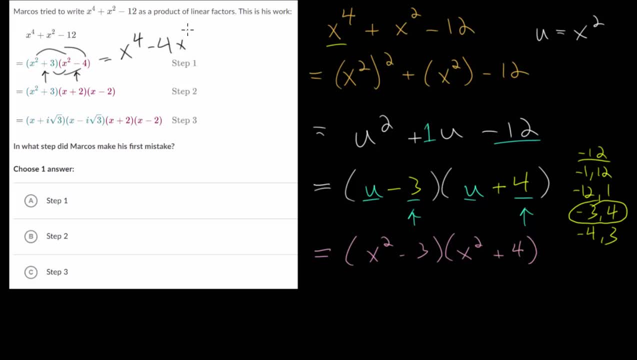 we would get minus 4x squared And plus 3x squared and minus 12 at the end, And when you recombine these you would get minus x squared rather than positive x squared. So it looks like the answer to our question here. where did he? 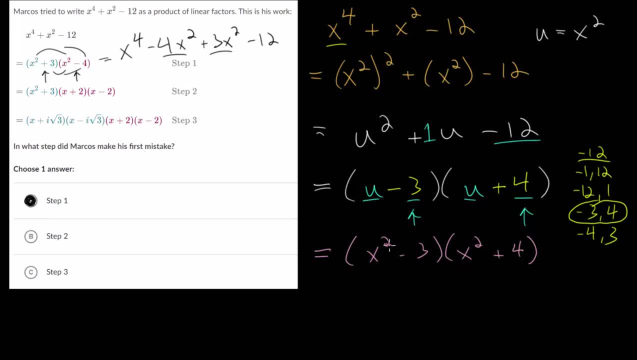 make the mistake is in step 1.. Now, if we wanted to, we can actually factor this further, just like he tried to do here. but he did it with this mistake in mind, so his final answer will be incorrect. But let's actually do this again. So, let's do this again. So let's do this again. 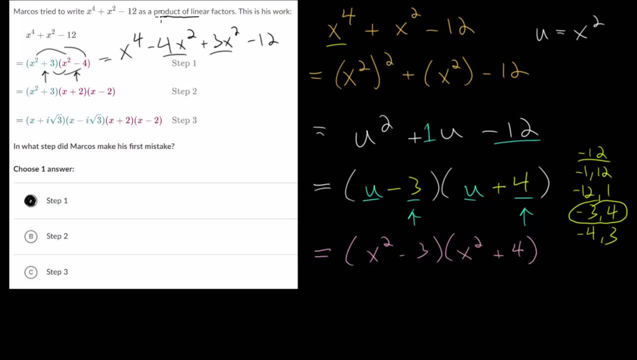 So let's actually continue this so that we can factor this as a product of linear factors where, essentially, we have x to the first power in each of these, And the key idea is to recognize that we have a difference of squares here and a sum of squares here. So remember the formula for: 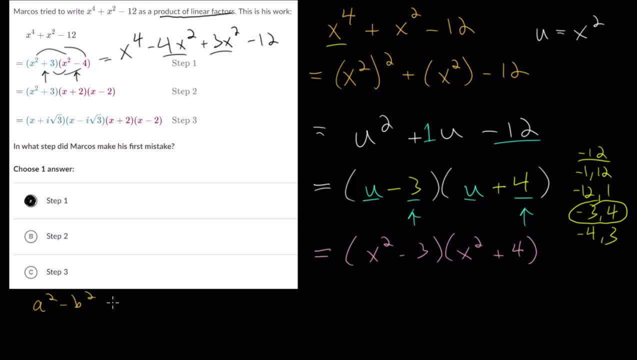 a difference of squares. If we have a squared minus b squared, we can factor this as a product of two binomials, where we have the first term minus the second term, And then we have the second term minus the second term, ignoring the squares, and then the first term plus the second term, And 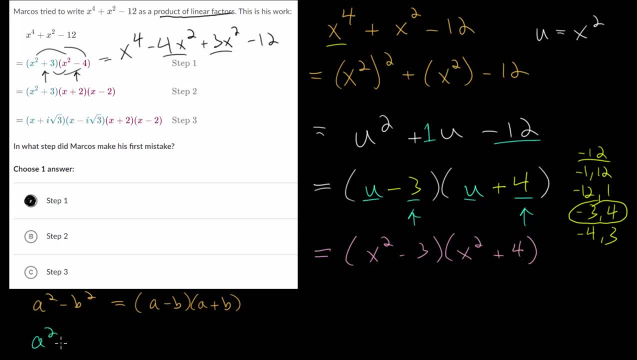 when we have a sum of squares. we looked at in a previous video that this can be factored using complex numbers. In fact, we can rewrite this as minus negative b squared, And just remember that since i is the square root of minus 1, i squared is negative 1.. And in that, subtracting negative b. 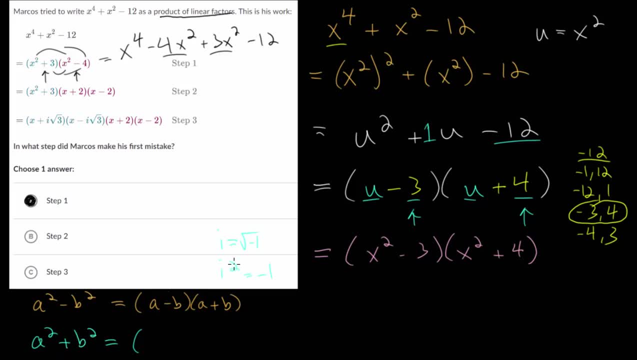 squared, we get a sum of squares. So let's do this again. So let's do this again. So let's do this again. We replace that negative b squared with just i squared times b squared, And then we can apply the difference of squares formula to that. But the result that we get is we get the first one.